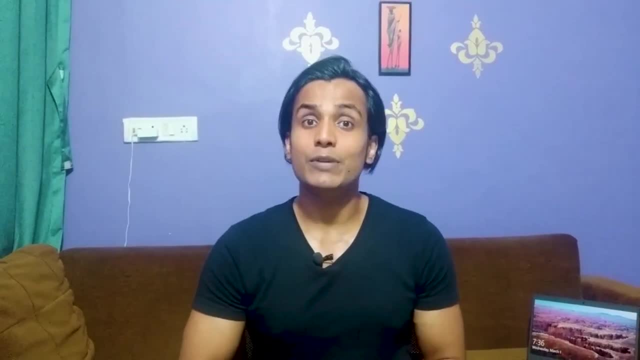 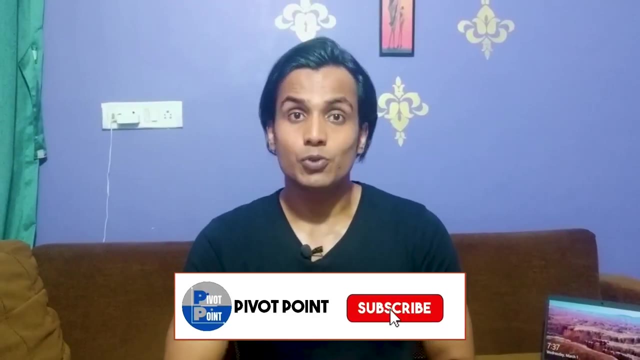 everyone Also packed with lots of values and information, and it will be really helpful for you, especially if you're preparing for a machine learning based job role like data analyst or data scientist. So please subscribe to the channel and drop a like below to support our work and. 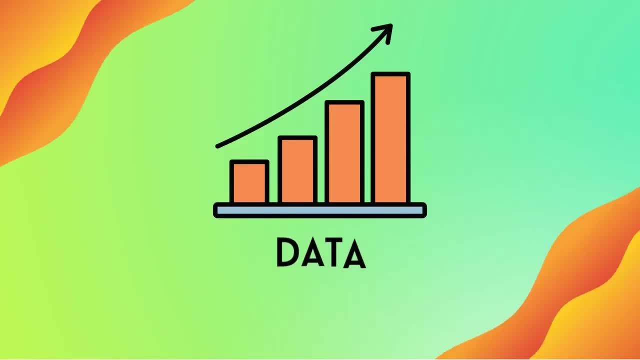 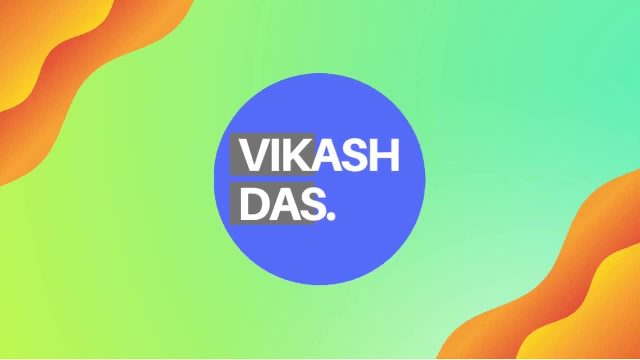 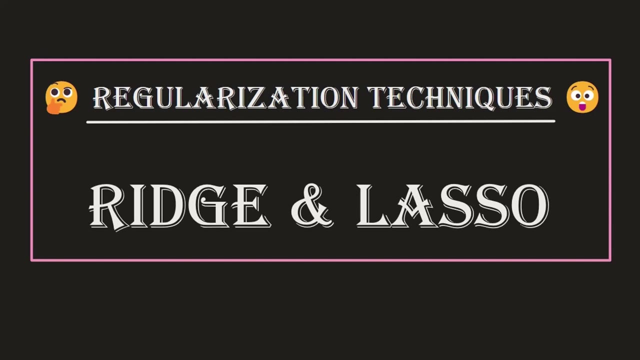 without any further delay, let's get started with today's topic. So today we are going to cover ridge and lasso regression. It is one of the most important topics, especially for the interviews, and I can tell this with experience because all the interviews that I 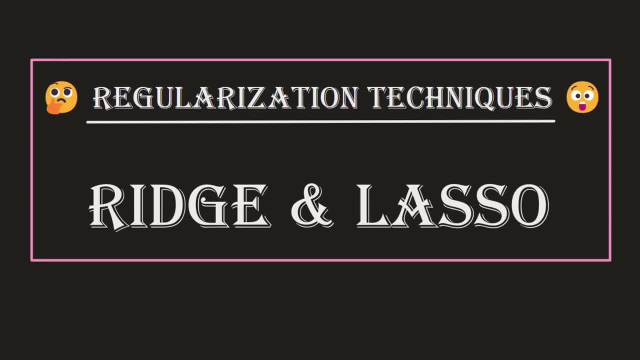 have attempted so far in my career, this topic has been asked. in at least 80% of those interviews They will either ask you directly for ridge and lasso regression, or you might be asked to explain the regularization techniques within machine learning, or you will be asked that how will you tackle overfitting? 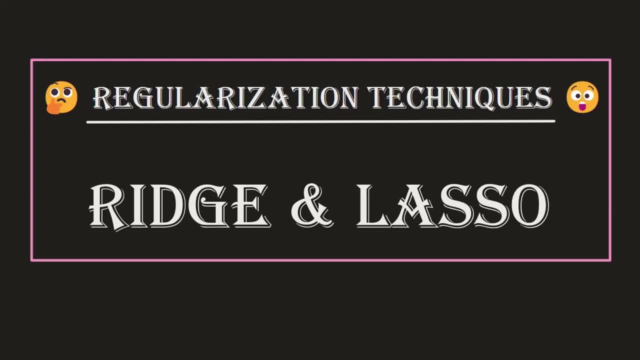 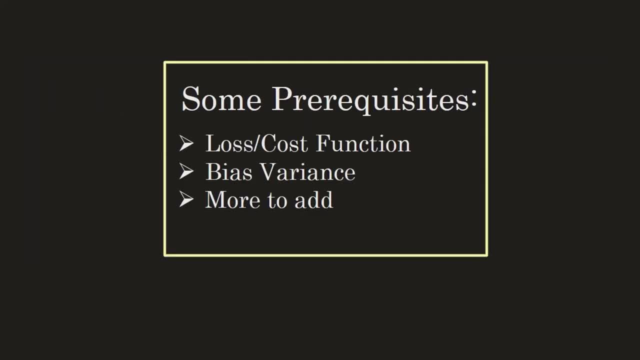 in your model? and the answer for all these questions will be a good explanation for ridge and lasso regression. So let's try to understand them one by one. Right before we get started, you need to have some prerequisites clear. Be sure that you have. 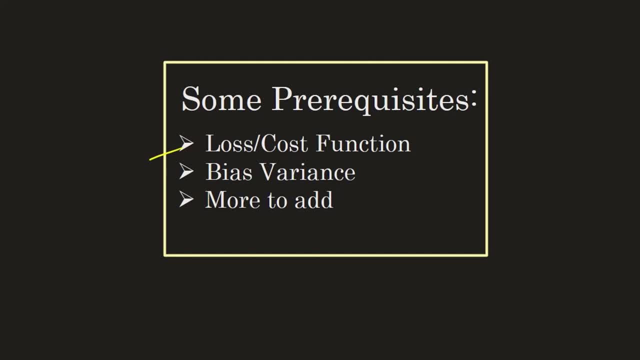 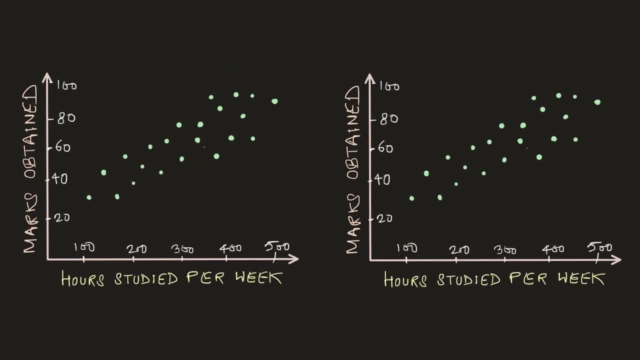 a basic understanding on loss function or cost function. You should be familiar with the bias, variance, trade-off and rest. we will cover within this lecture itself. So, in very simple words, ridge and lasso regression are nothing, but they are regularization or hyper tuning technique. that 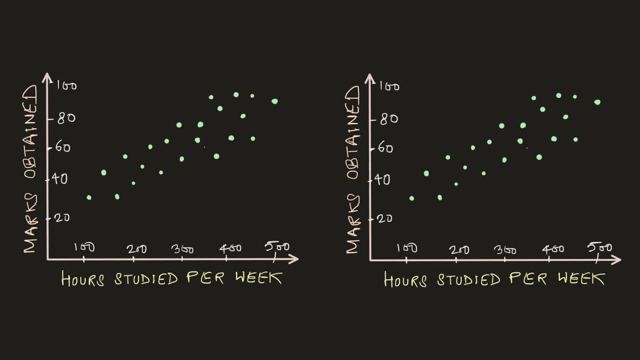 helps us to prevent overfitting in a model and additionally, it also helps us with feature selection, and we will see how. So we are already aware that, in general, within a regression model like linear regression, all we want to do is try to adjust the slope and bias in such a way that we 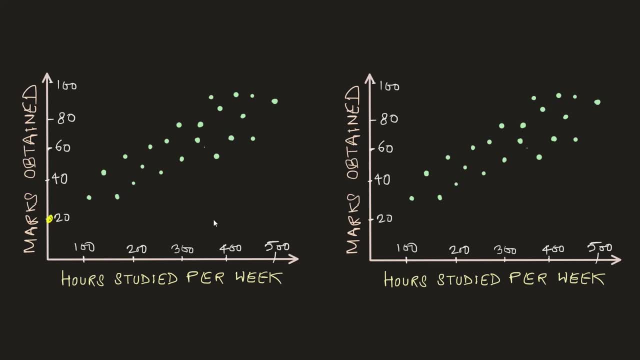 achieve the minimum value of a cost function. So we try to keep the bias and the slope of the straight line in such a way that the value of the cost function or the loss is minimum, which is nothing but actual value subtracted by the predicted value and then the summation of all the 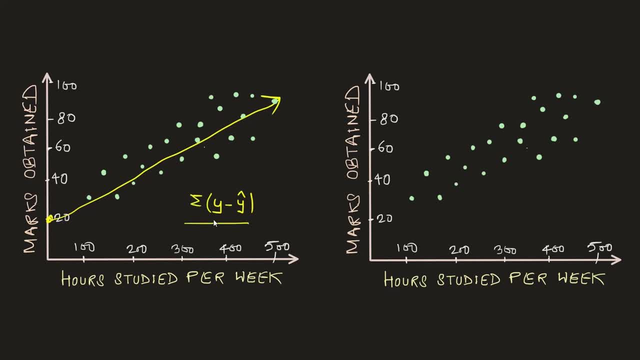 records. Let's say, for simplicity purpose, that this is the cost function that we try to minimize. So it is just an imaginary cost function and all we are trying to do is to minimize this cost function as much as possible by drawing straight lines. However, this intuition might lead to overfitting. sometime I'll tell you how. 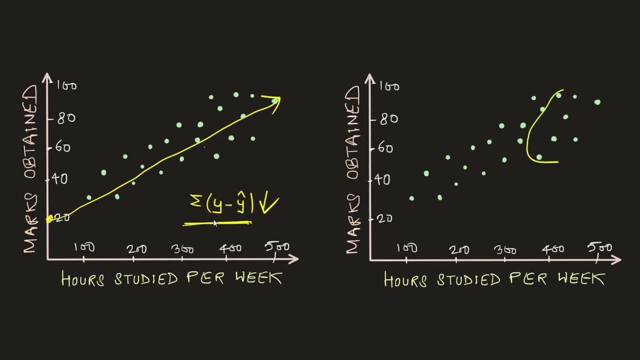 So let's say that we are keeping this part of the data set for testing purpose, which means after drawing the straight line or the best fit line, we will try on these data points that if our best fit line is performing well or not. So we are using only leftover data points over here. 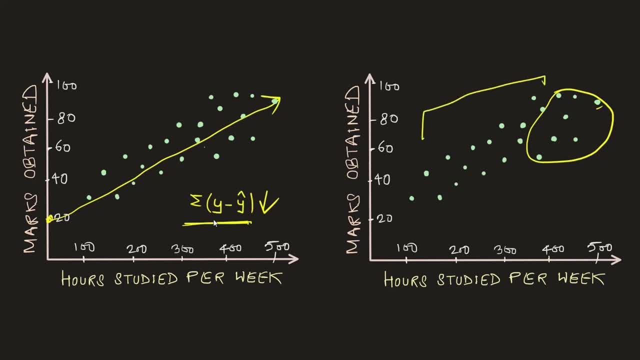 within this range in order to train the model, or you can say, in order to draw the best fit line, And let's say we are drawing the straight line like this. Okay, Of course, this line is performing really good with respect to this training data, and the loss as well, is very 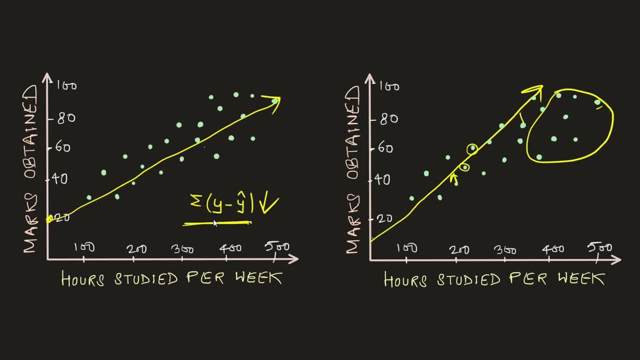 less. So there is a minimum loss and the entire cost function is probably pretty much less. But what if this same straight line is being tested on this test data? Then it will perform really poor. You can see the loss has started increasing, which means it is the case of low, bias and high. 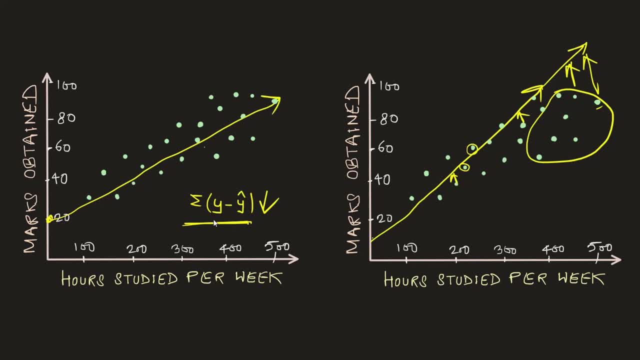 variance which is nothing but overfitting. And this is where ridge comes into the picture. So let's try to understand first visually that how ridge is preventing this overfitting issue. So within the technique of ridge regression, we don't only focus on achieving the minimum loss. 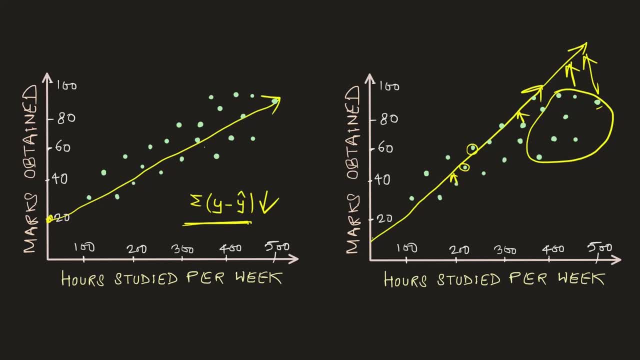 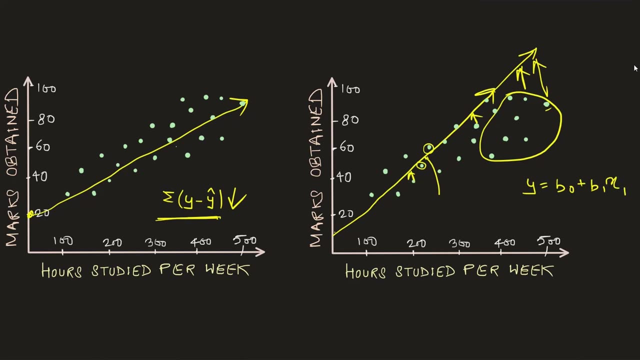 by adjusting our weights. but we also focus on avoiding a steep slope to tackle overfitting, Which means if the value of this slope, which is beta 1, within the equation of, let's say, y is equals beta 0 plus beta 1 and x1.. If the value where beta 0 being the bias over here, and beta 1 being 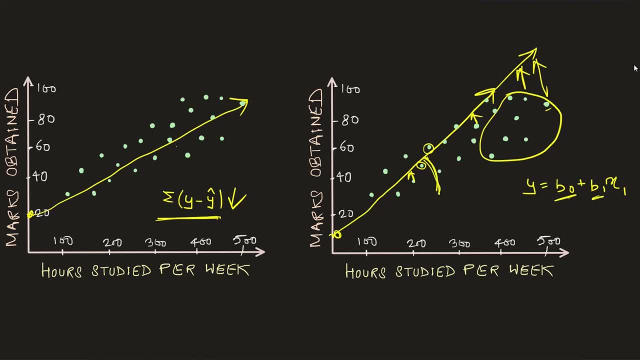 the value of the slope. If this value is too much, which is leading us to have a steep slope, in that case, ridge will penalize the model and it will try to decrease the value of this slope so that we can have a straight line that also performs well with the testing data. Now let's 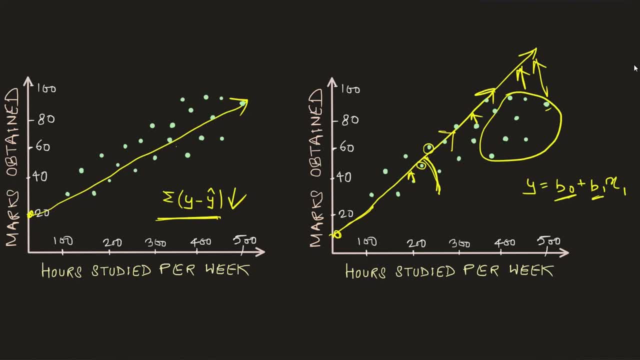 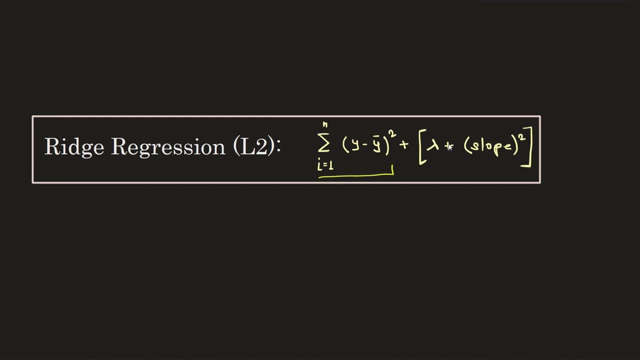 have a closer look on ridge regression to understand better. So let's see how exactly it is doing that. So it is the formula for the ridge regression, where it is definitely focusing on minimizing the loss. So over here, the loss function which is used. 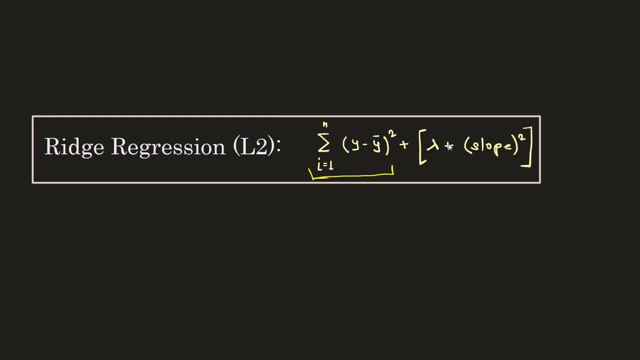 it is mean squared error. So we are doing nothing, but we are taking the difference and then we are squaring it up And additionally, we have this term where we are squaring the value of the slope and adding a small lambda value term over here. And in general, what we are doing is instead of 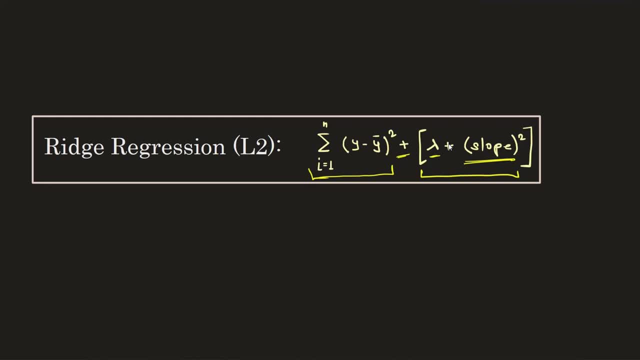 trying to minimize the standalone loss function. we are trying to minimize this entire thing over here. So if the value of the slope is increasing, the ridge regression will penalize the model in order to have a generalized slope that can perform well with the testing data as well, along with the training data. As simple as that. 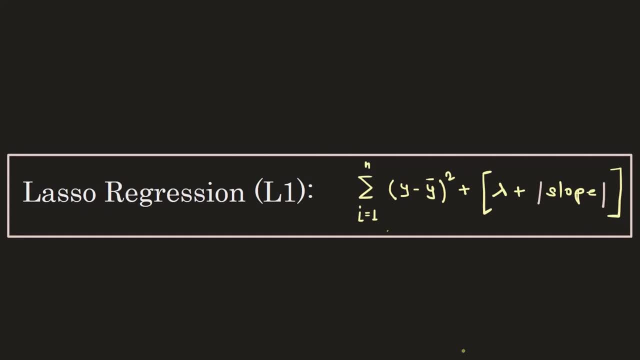 And the formula for lasso regression is slightly different and what it is actually doing is: lasso helps us to discard the feature with very less magnitude, So it helps us with feature selection and it helps us to reduce the overfitting. So let's say you have one dependent value, that 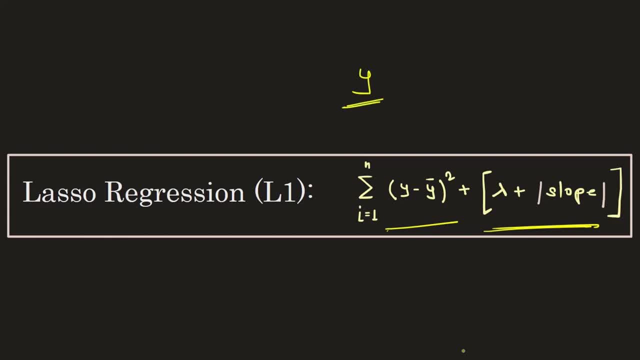 you are trying to predict- Let's say it could be price of a house or something- and you have few independent variables, like, let's say, a, b, c, d. Okay, let's say you have four independent variables as well. In that case, let's say variable a is contributing a lot to predict the price of the. 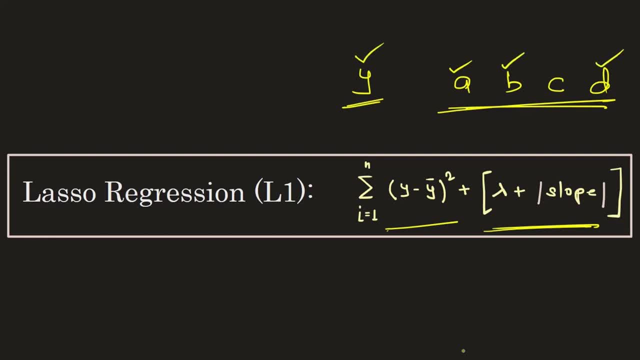 house, B is contributing a lot, D is contributing a lot, But c is not contributing. that Let's say a is the number of bedroom, B is the number of bathroom, D is the area of the house. And let's say c is the number of trees nearby the house. Okay, that. 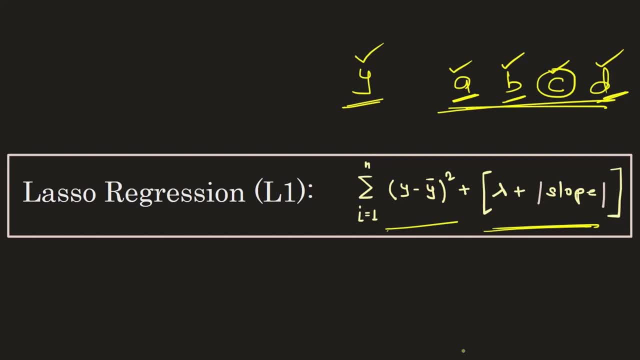 how many trees you have nearby the house. So this feature is actually not that important in order to predict the price of the house, And lasso regression is efficient enough to detect that. So it will simply discard it. It will simply discard this feature so that our model doesn't get. 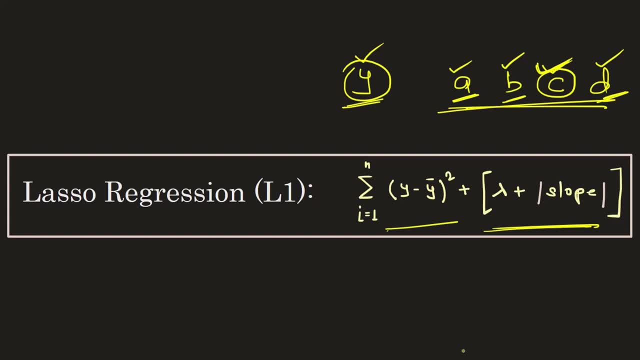 confused And, along with tackling overfitting, it helps us with feature selection as well. And this is a very simple and basic explanation on ridge and lasso. Trust me, if you are able to give this much explanation on your interviews, it will be more than sufficient for you. So next time you. 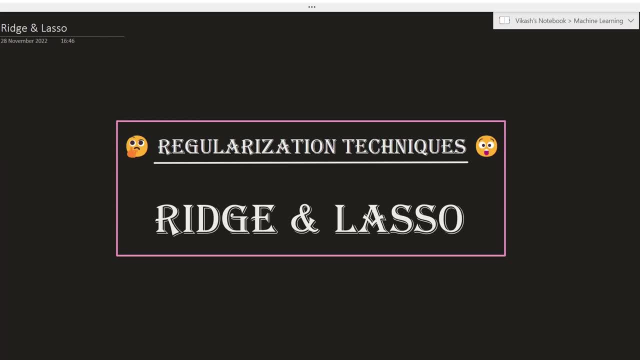 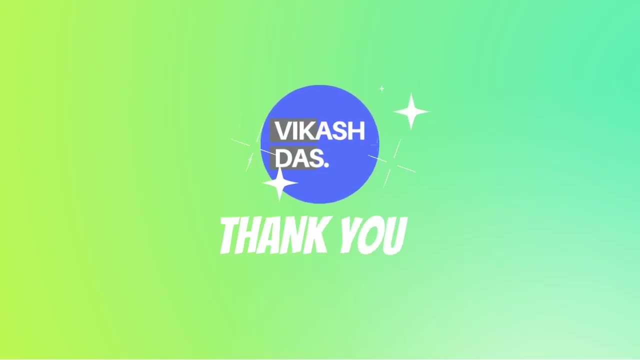 come across a question on elaborating some regularization techniques or what is your approach on handling overfitting. You can give a straightforward explanation on ridge and lasso regression. Thank you very much for your time today you.